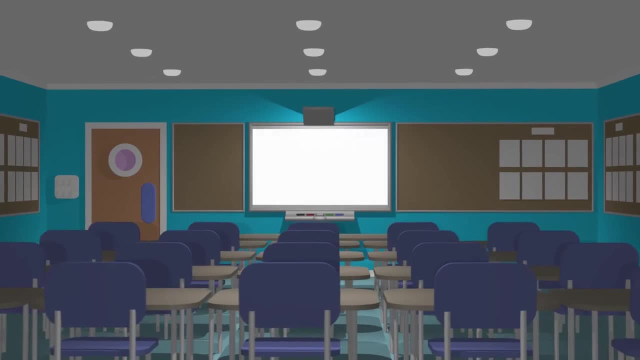 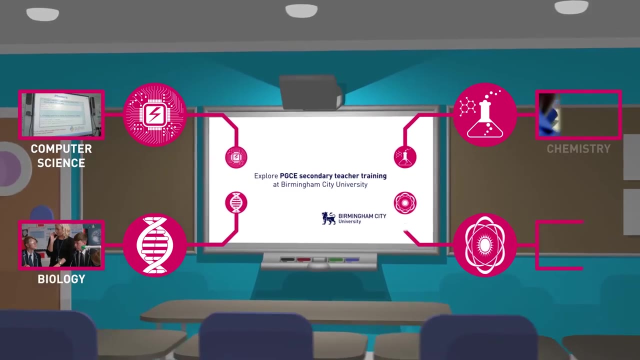 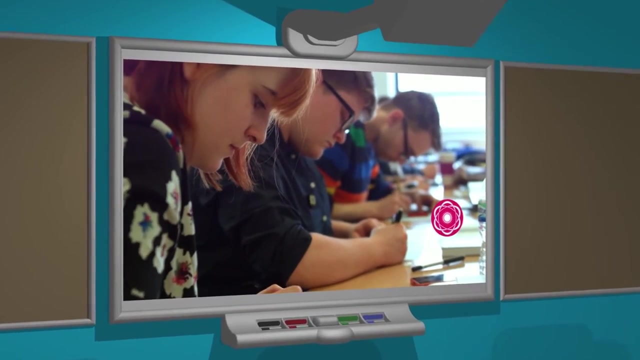 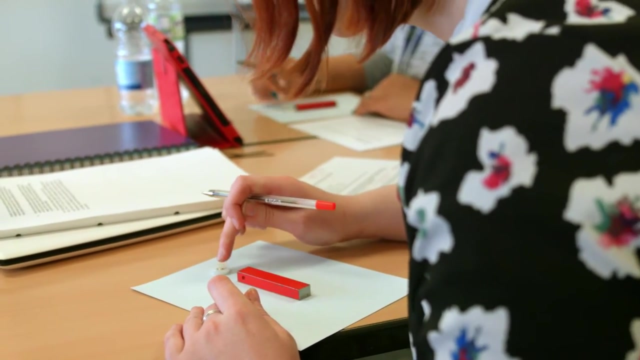 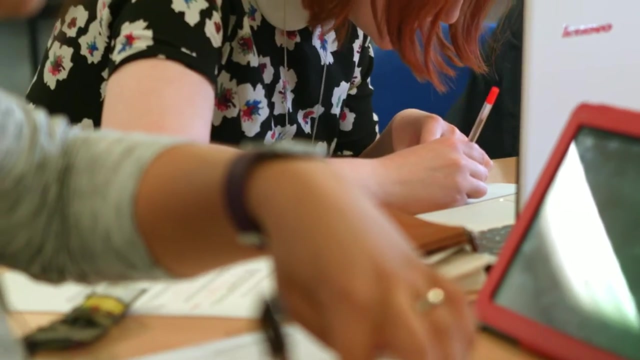 Then move the plotting compass out so that the other end of the needle is by the point and then put a dot at the other end. there I'm studying science with a specialism in physics. Science as a whole, I think, is a fascinating subject, and physics really just underpins. 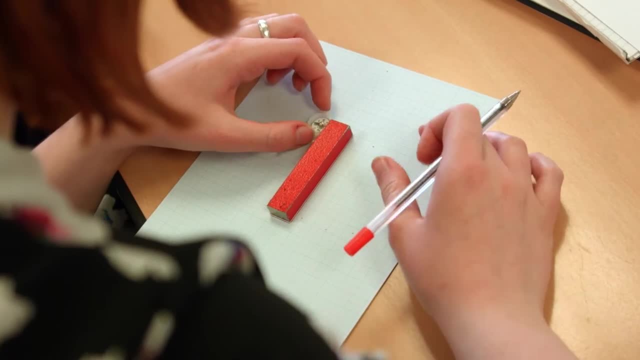 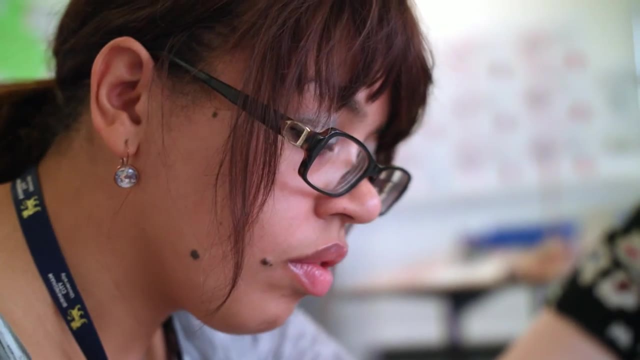 all of them. It really helps you understand how the world works, and I think that's something that it's quite easy to be passionate about and to sort of pass that passion on to the kids. I'm studying PGCE science with a physics specialism. 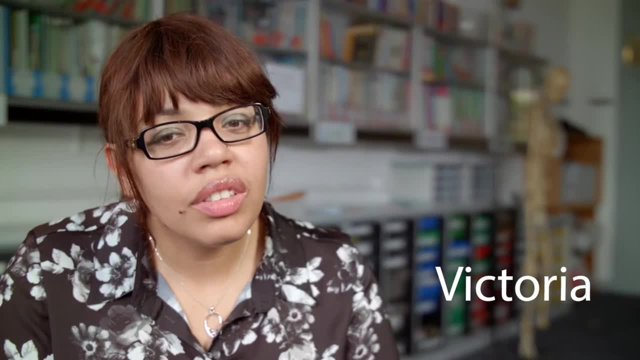 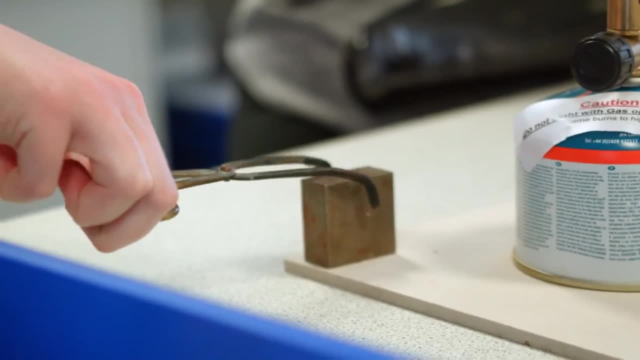 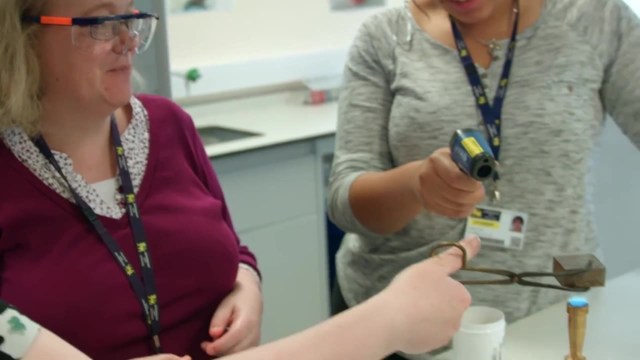 I'm fascinated with how the world works, the physical processes behind it, The enquiry methods that we use to discover, and I want everybody to love it as much as I do. If you put the infrared gun on to that, what sort of temperature have we got? that iron? 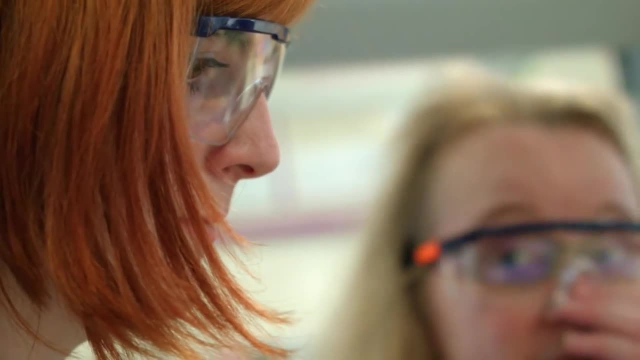 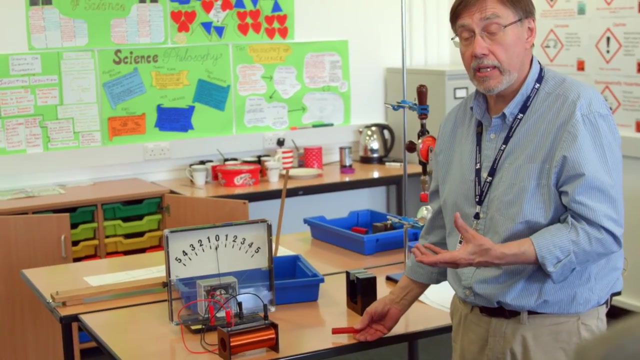 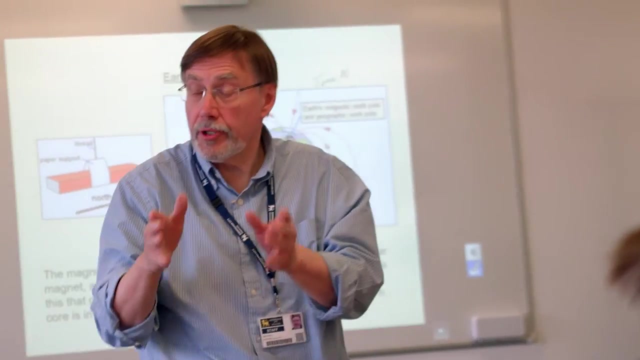 out now. Okay, 151.. The lecturers are very engaging with their teaching and the tutors are very empathetic, they're very supportive And you must emphasise to pupils, when you're doing this, why it's called a PhD. It's called a North Pole, it's a North Seeking Pole. 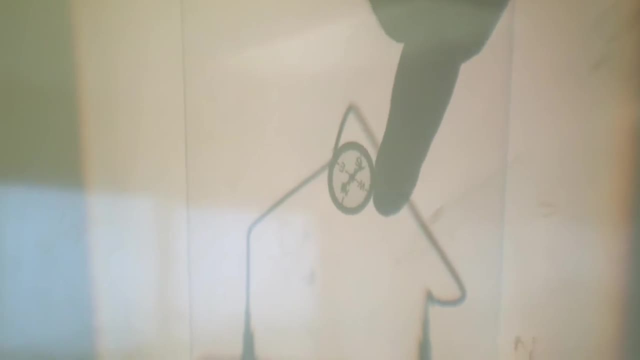 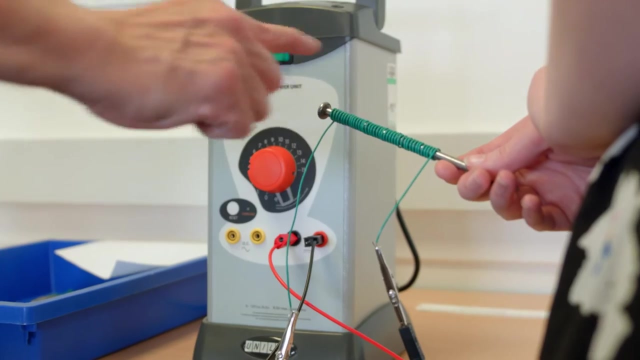 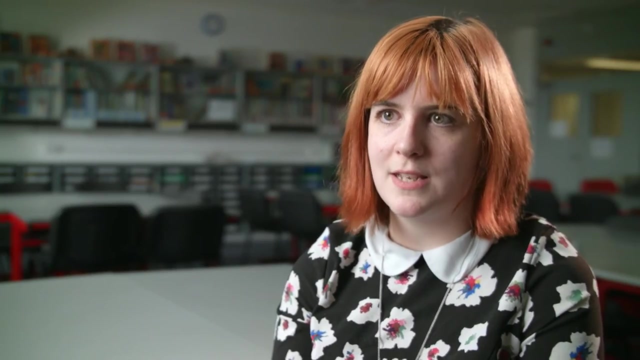 We have seminars and workshops where we really get to grips with the pedagogy of teaching physics. We use what we do in university within the school placements. There's so many different things you can do. It's not sitting in a classroom talking to the kids, it's. we're going to talk about this. 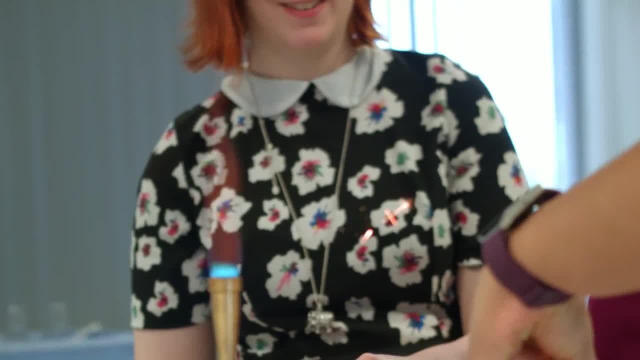 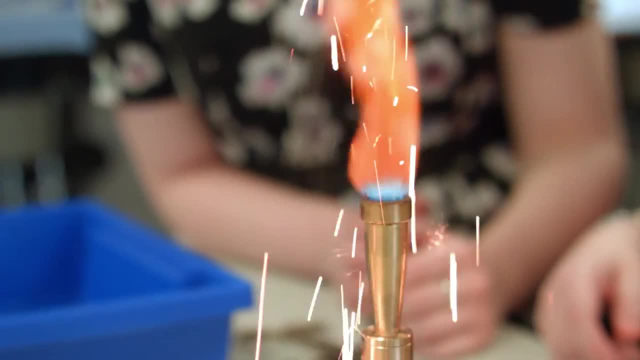 today. look now, I'm going to show you it. And it's very physical, it's very tangible. you can show them how the world works on a miniature scale, So you could actually have a little mini assessment at the end, where they go back and write a. 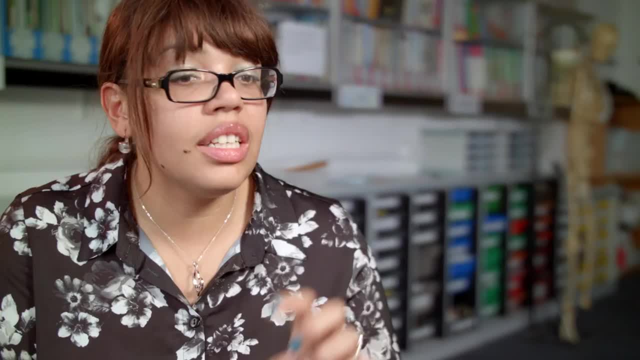 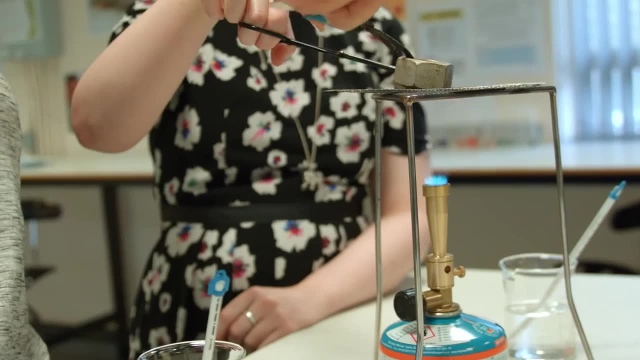 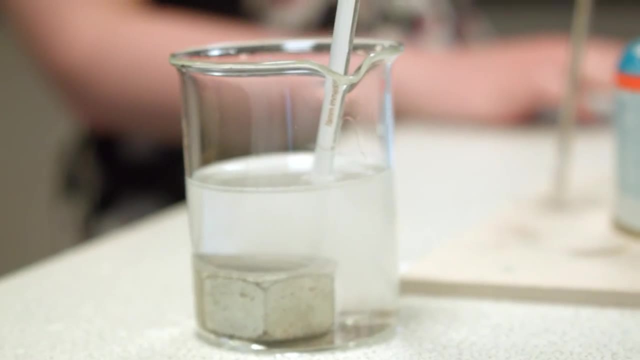 few sentences. Every child is a natural scientist. every person can do physics. they can do science, and I want to facilitate that and I hope that I do it in a way that's engaging and fun for them. It's like this is what I should be doing.